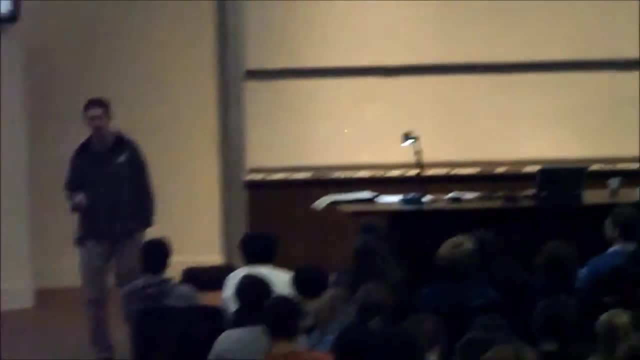 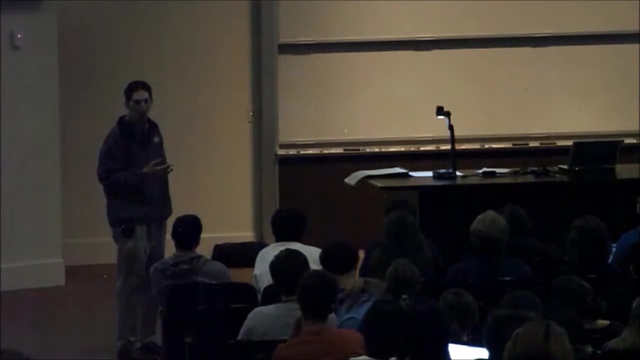 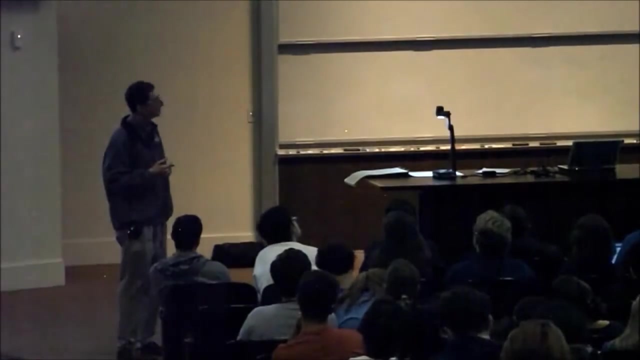 and it's a particle. don't know why. that's just how the universe works, So we can explain it either way. The wave explanation's kind of complicated. You have to follow the wave and follow how it diffracts off of every particle in the medium, in the glass medium. 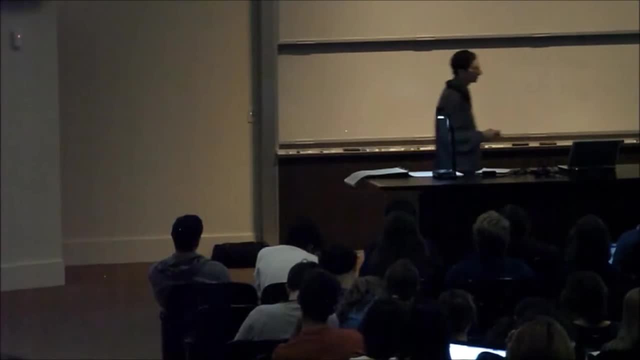 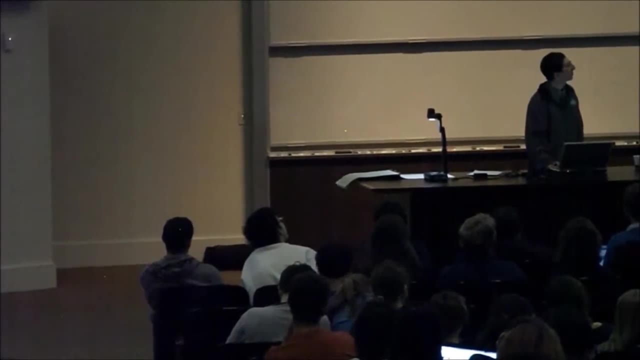 The particle explanation. Newton's explanation is a little easier, so I offer it as a cartoon picture to keep in mind. It'll also help you figure out which way the light will bend as it transitions from a medium in which it moves easily to a medium in which it has a 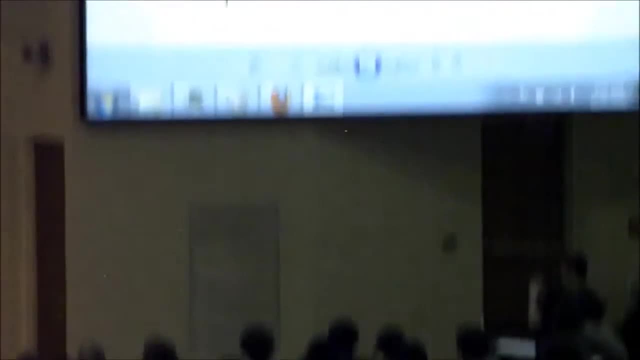 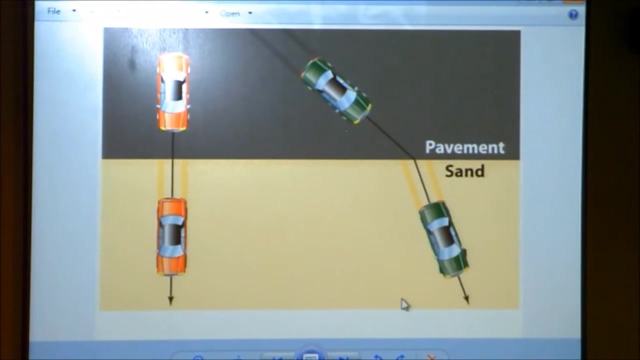 harder time moving. So envision your light wave as a particle. This is again Newtonian-type explanation, and we'll envision it as a car going through an easy-to-move-on medium such as pavement into a difficult-to-move-in medium such as sand. Anyone ever drive your? 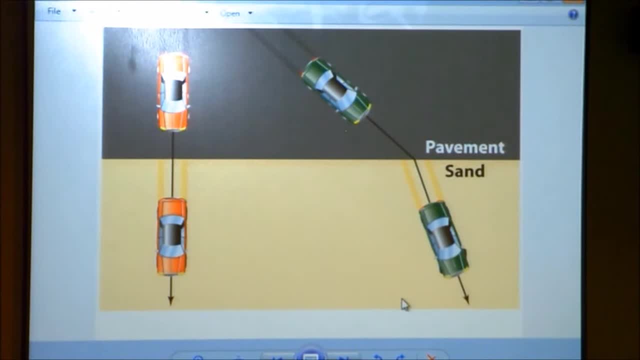 car on sand, Did it not work? Yeah, not well, I learned that one the hard way. Anyway, you go straight in. you'll keep going, at least until your wheels get stuck, But you know if you're driving the right vehicle. you can of course do it, But my Ford Tenpo is not. 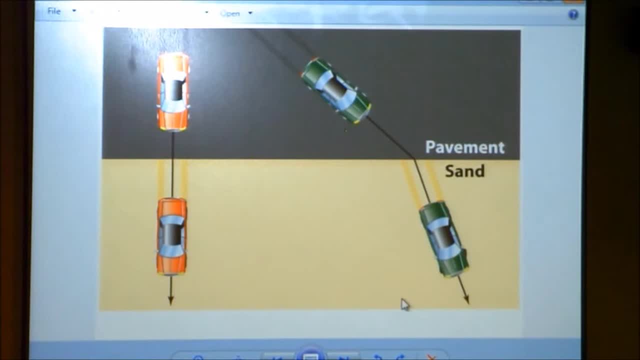 the right vehicle Moving in at an angle. we've got two wheels up front. We have the driver's side and the passenger's side. The passenger's side's going to hit the sand first. It's going to have a harder time moving through that. medium Light has a hard time moving through glass. 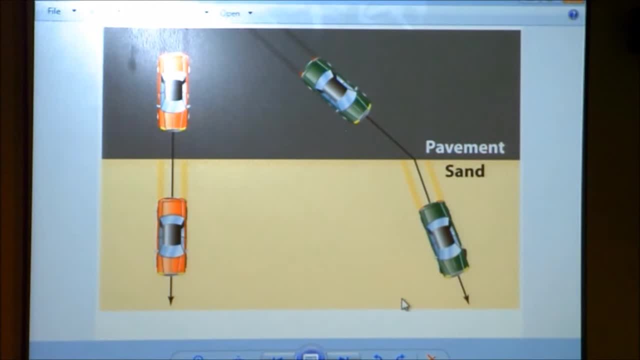 just because it's going to scatter and diffract off of all the atoms in the glass. It slows it down, takes a longer path, But here, with this analogy with sand, the passenger's side wheel will start moving slower, But the driver's side wheel is still moving quickly and that's going to give you a change. 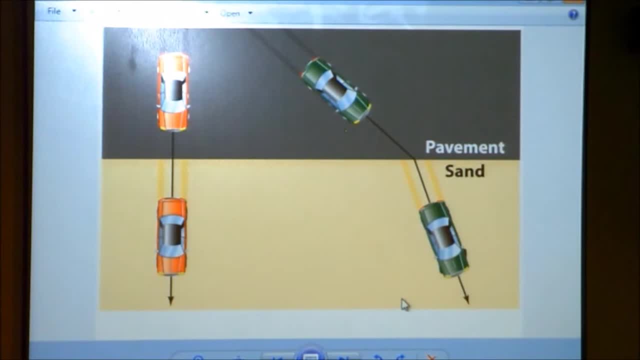 in your trajectory. So as you transition from the pavement to the sand, your car would actually change its direction of motion. That make sense. You can see that intuitively. So it works the same way for light, except it's a more complicated wave phenomena, but same. 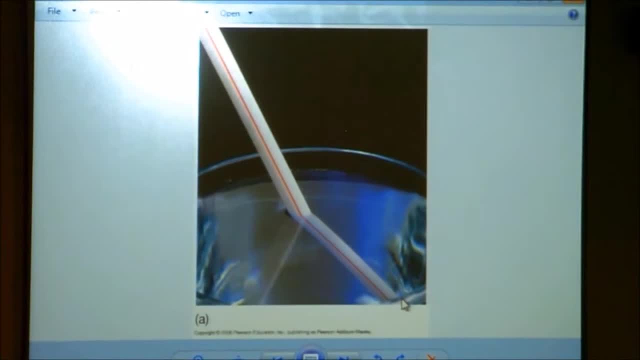 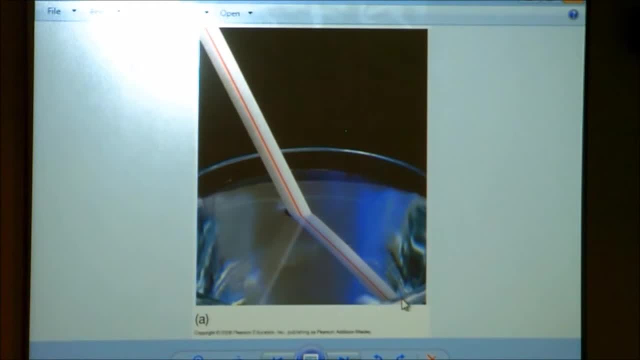 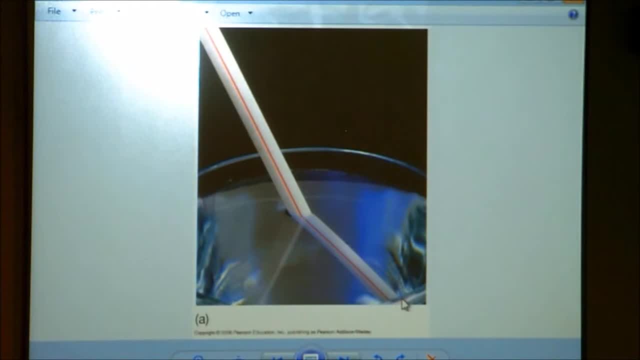 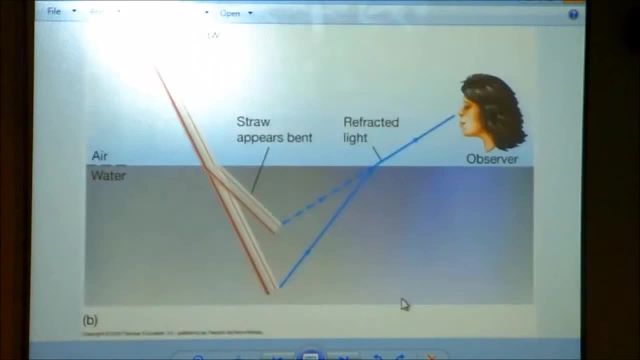 to not have realized it. But yeah, you look at the straw and you say: wait man, I know that straw didn't bend when I stepped into the water. it's an optical effect, it's refraction. Here's what's going on. Here's the straw. it's actually going straight into the water. 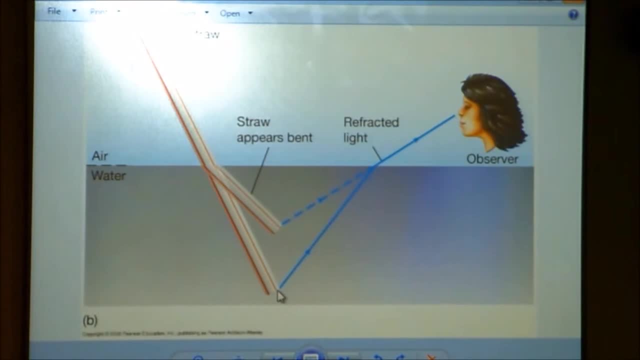 just as you think physically, Here's the light coming from the very tip of the straw. It's heading off in all directions. So the light's going up in all directions. this way, some of it's going this way, but let's take a particular path. coming from the 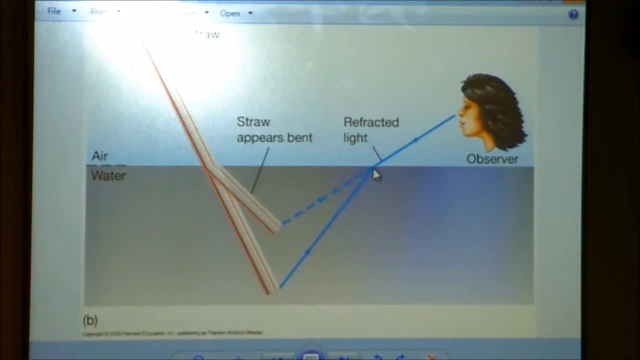 tip of the straw out in this direction. Then you're going to transition from, in this case, water to air, the denser medium to the less dense medium. So again, envision it as the car leaving the water medium. You have the front two tires, In this case the driver's. 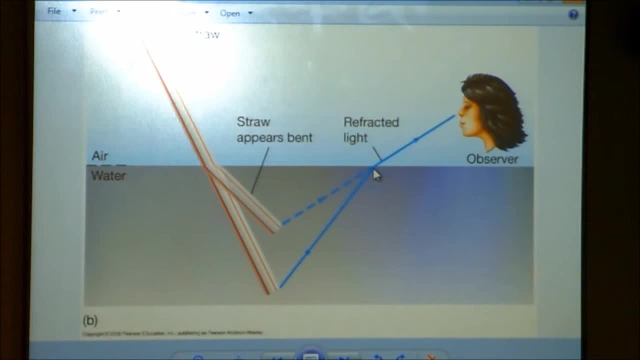 side tire is going to transition into the easier to move through medium more quickly. You can envision it as the driver's side tire going from the sand to the pavement. It's going to have more traction. It's going to bend the car, So in this case, the light. 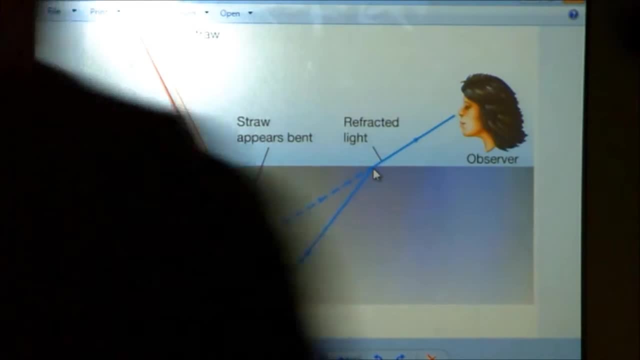 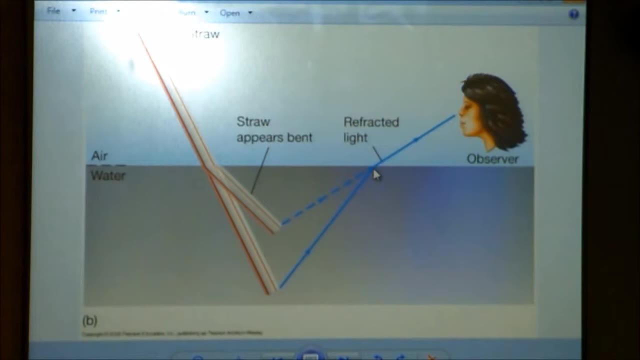 wave is going to bend off to the right and in this case go into the observer's eye. But the human brain, your visual cortex, it doesn't do diffraction calculations. So the brain is going to assume that the ray is coming straight from where it was emitted. It doesn't. 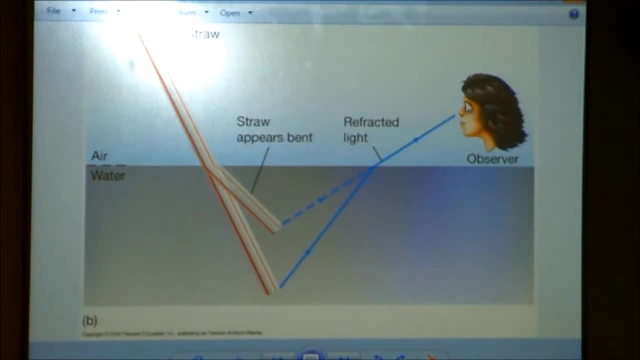 know that there's a density difference between this medium and this medium. So if we follow the ray, it's going to assume that the ray is coming straight from where it was emitted. So if we follow the ray's path back out here, your brain sticks to the tip of the straw. 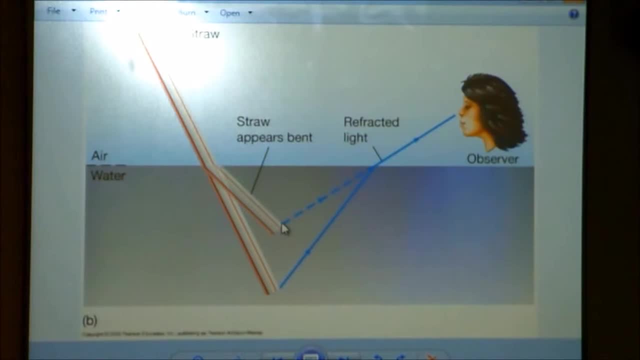 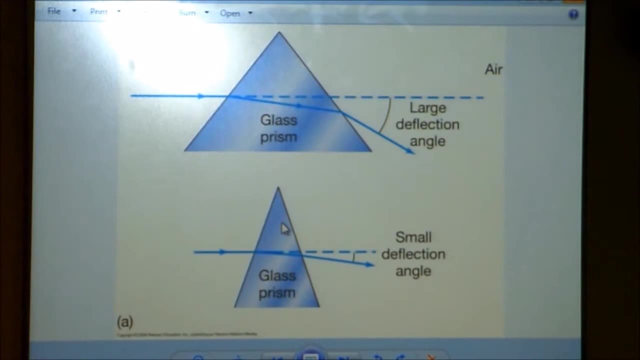 there. That's why you see kind of a bent straw. Make sense, Okay. As for traction, let's start considering light again going through glass, because that's what we typically use to make lenses. Instead of starting with lenses, let's start with something simple like a prism. 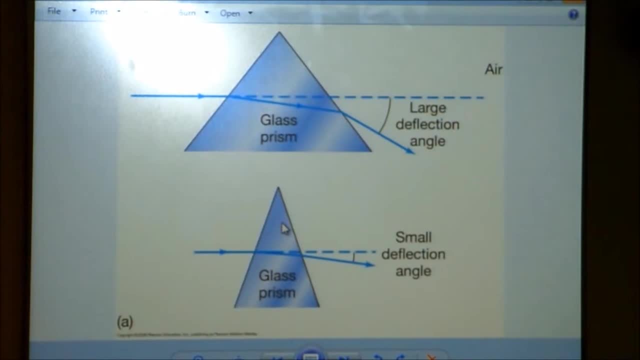 I've got pictures up here. I have a big prism here. I'll use it in just a second. So again, we can just envision this as the car going from a pavement to sand medium or an easy-to-move-through medium to a difficult medium. Here we have a light. 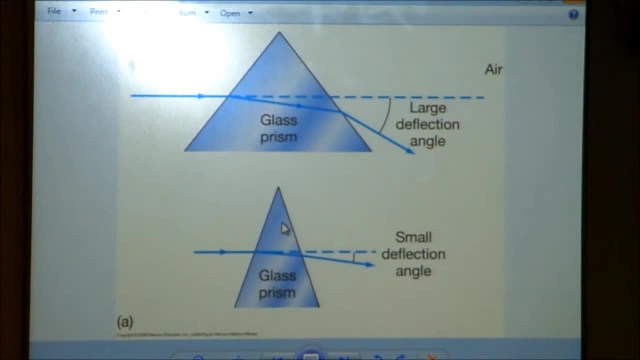 ray going straight into the prism. The glass is at a tilt, though If it was going straight into glass head-on, it would go straight in, as we've talked about before, If we go back a few slides. I'll just point that out one more time. If you go straight into the glass, 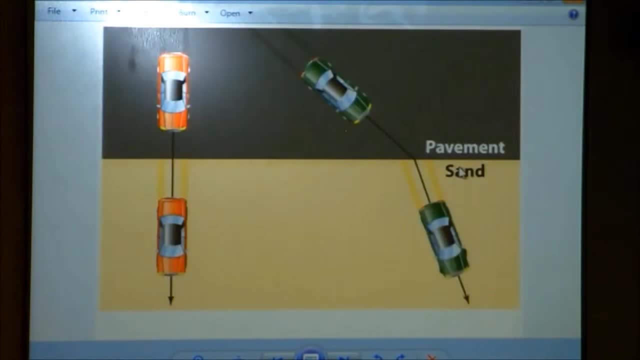 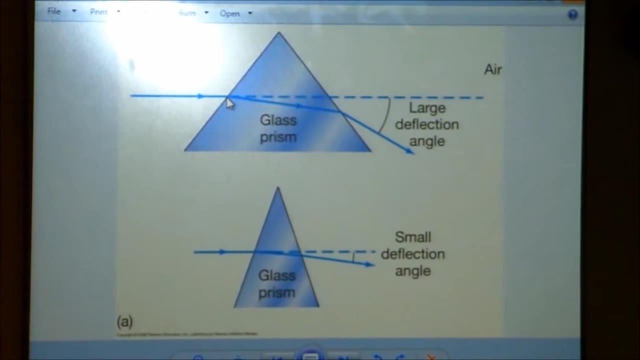 the light goes straight, But if you come in at an angle with respect to the glass surface, you'll refract. So that's what we're doing here. Here it's coming to the right, but it's not impacting the prism straight on. 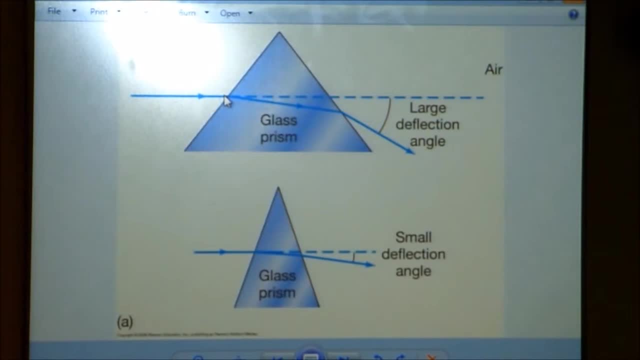 The glass surface is at an angle, and so you're going to refract. In this case, the passenger side wheel gets into the more difficult-to-move-through medium first, so it's going to bend, in this case, down. The driver's side wheel is going to keep pushing and change the angle. 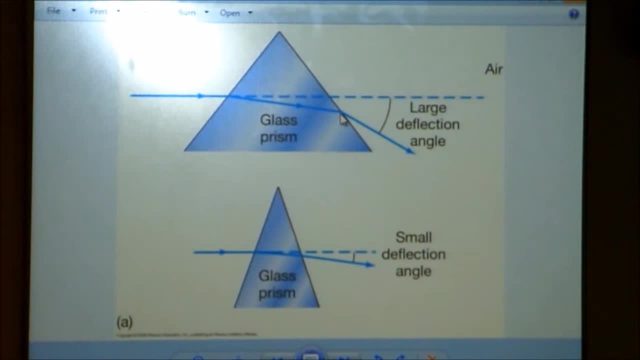 and it's going to continue out until it hits the other side of the glass. And again you've got to think about the two wheels. The first wheel out will be the driver's side wheel, so it's going to turn the car again in the same direction, giving you kind of a large 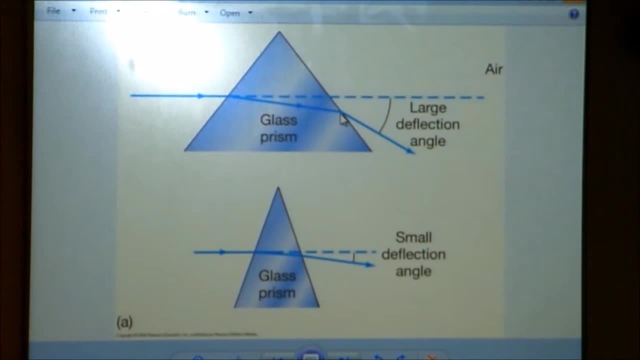 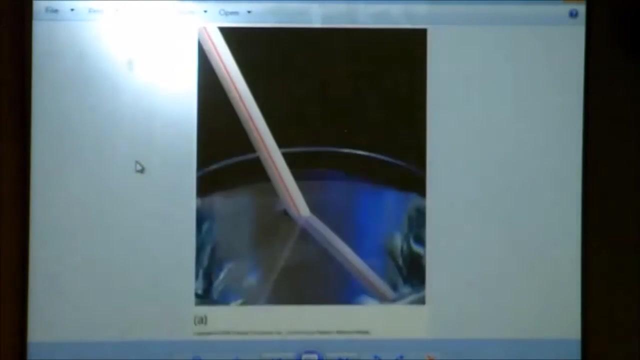 deflection angle From where it was going- the dashed line- to where it is now going. Now, if you go through a skinny prism, the same thing happens, but you're closer to hitting the glass square on Again. if we come back here, we go into the glass directly without any angle of incidence. 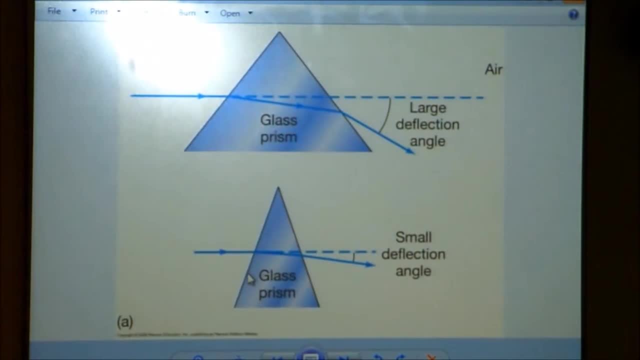 other than head-on, you're going to have less refraction. So here with the small angle prism, it's closer to hitting it straight on and you get the same effect- just a small deflection angle. So let me demonstrate that here. 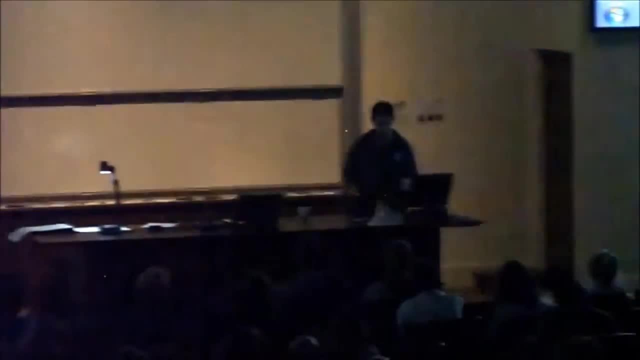 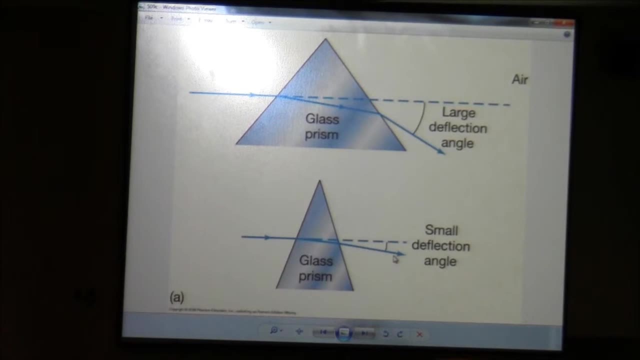 You can very easily build up the concept of a lens from the concept of prisms. I've brought up a big prism and a laser. I'll turn the lights off and we'll see if we can make this work. Lights all off, Okay. so let's see, I've got the laser. There it is, It's. 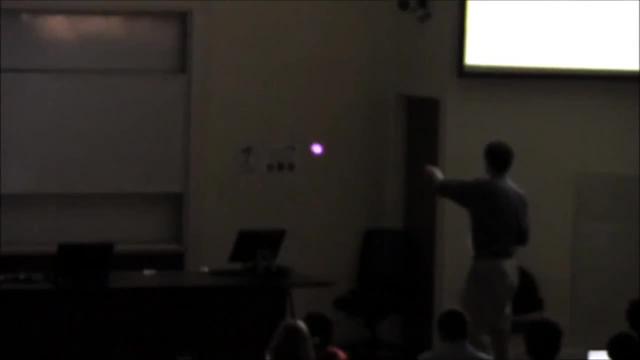 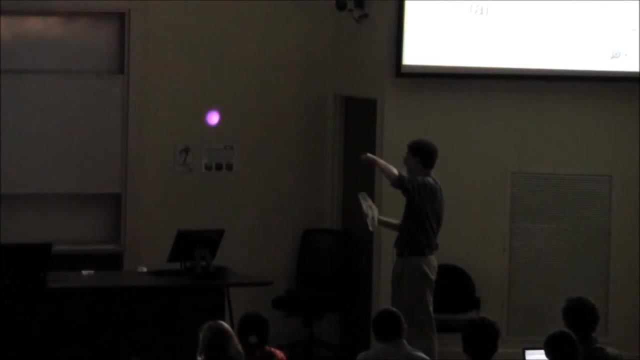 a purple laser today. Now I think I'll do the narrow angle first. This will be the lesser deflection. So if I hold it here and I raise the prism into the beam, it'll pop down lower on the wall Only. 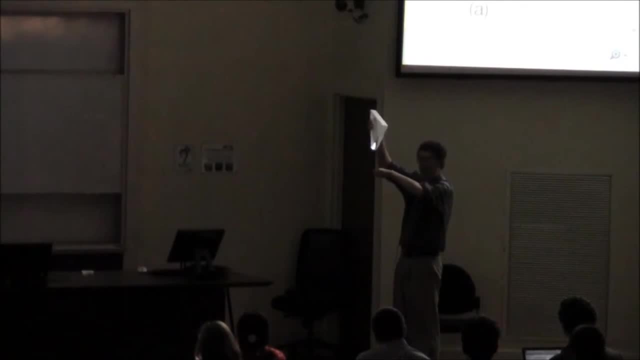 people in the front row can see that. So now I'm going to change it. I'm going to go in from above and we can watch where it goes. I'm going to try to keep my arm out of the way here. So there's the spot, and coming in from above, we get a small angle deflection. 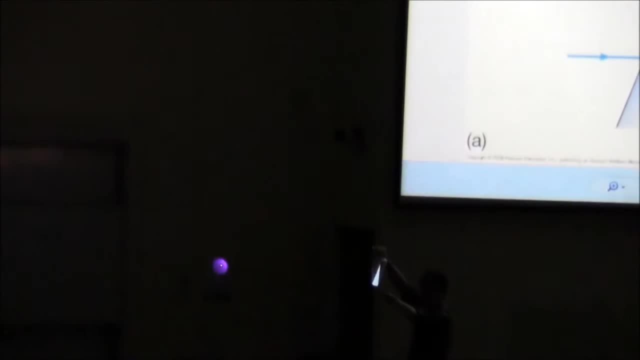 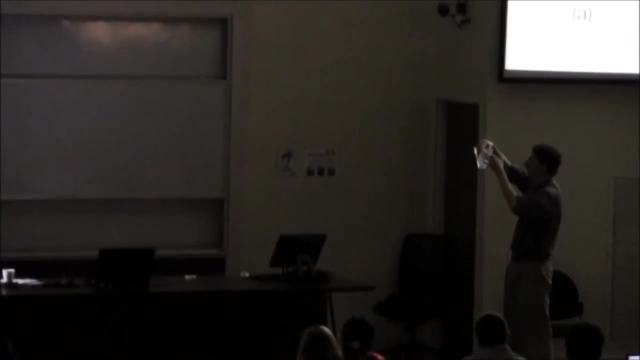 See how it popped up there. Everyone got that. Okay, now I'm going to turn the prism. this way You can make use of the wide angle part of the prism, and we should get even bigger deflection. I'll find the right place to hold it here. 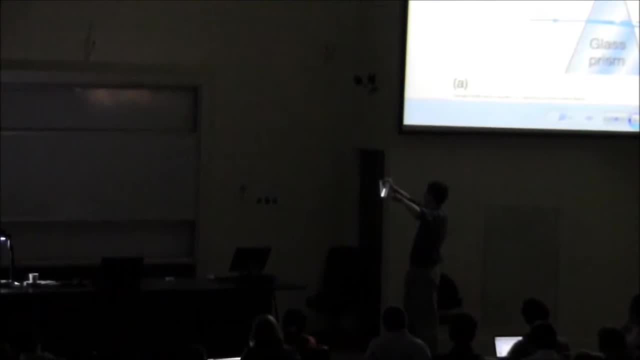 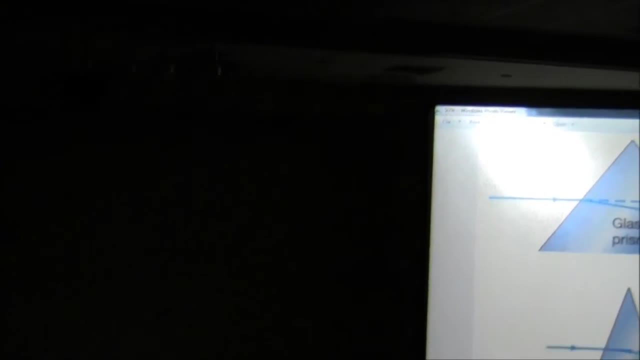 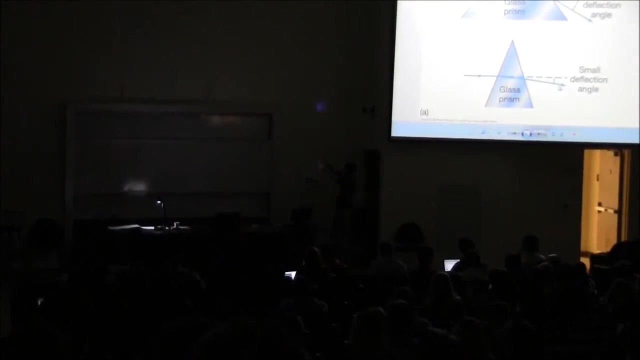 Okay, so there it is going straight and we have a wide angle deflection. And where is it? It's like way up there. I'll come closer to the wall so you can see the difference again. angle: so we get just a little deflection. Here's the wide angle. we get a bigger deflection. 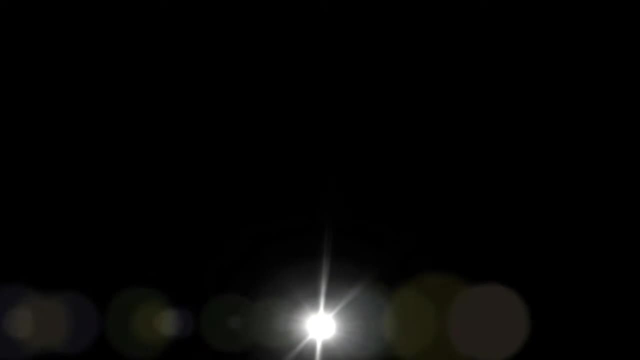 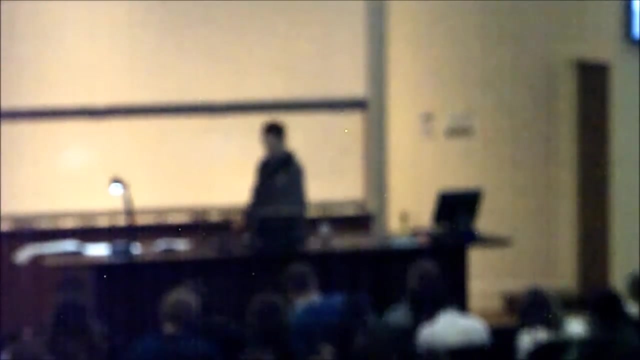 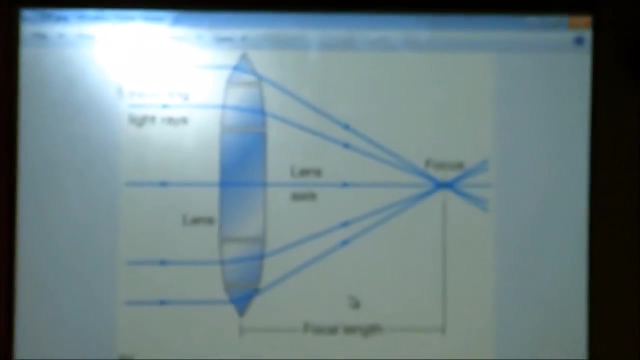 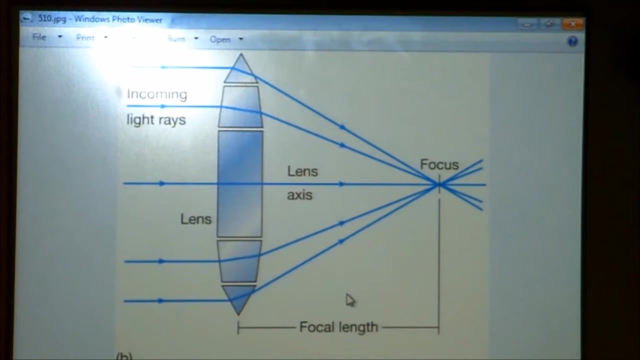 Good, Okay, Okay, we can make a lens out of a bunch of prisms. We now understand how light's going to refract through prisms of different angles. So what I have here are prisms where I've chopped off the top. Well, yeah, So at the very top I have just a regular wide angle. 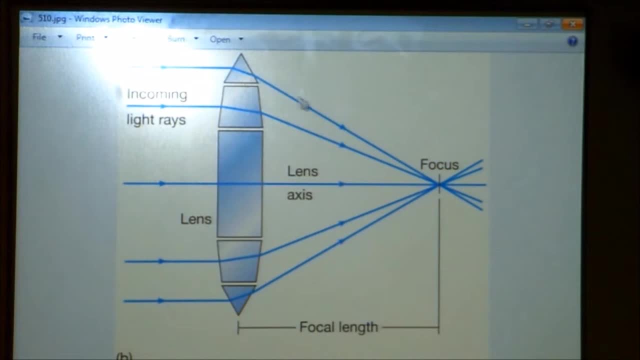 prism. right here Light's coming in. we're going to get a big deflection angle, send the light all the way down here to what will be the focus point of the lens. This right here. you might not realize it, but it's a narrow angle prism. I've chopped off the top. 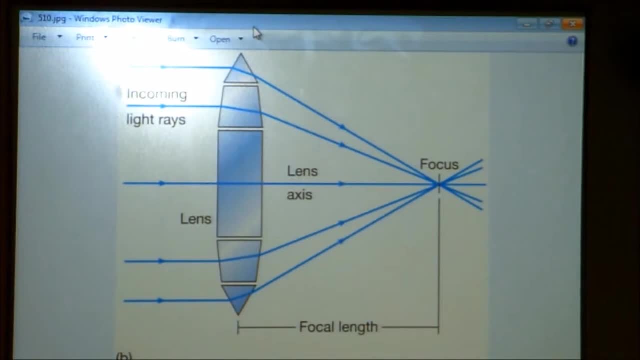 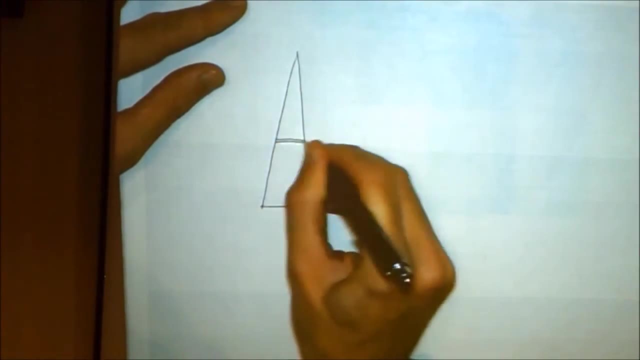 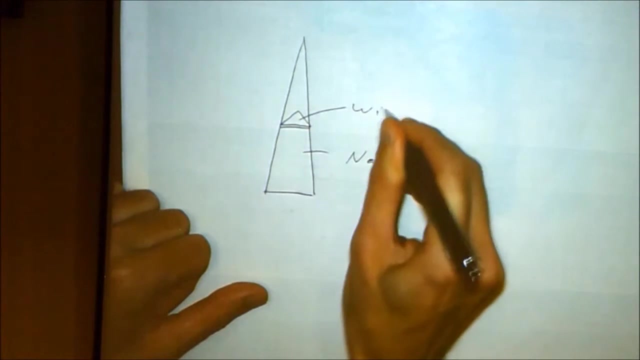 of it. but here's the basic idea. It's a narrow angle prism and it's just this component. And then on top of it- I've pasted this- I've attached a wide angle prism. This is wide angle, this is narrow, So we don't have 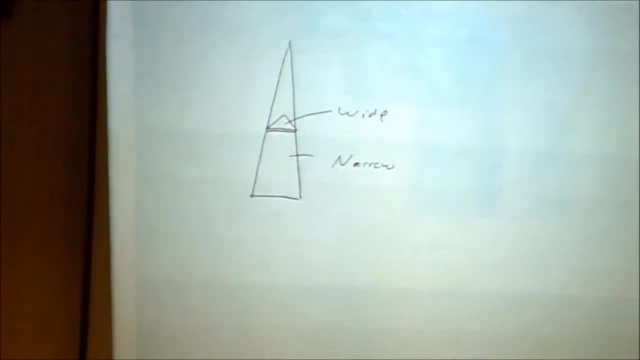 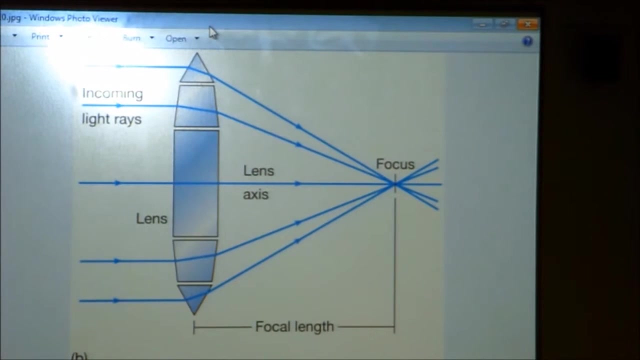 the whole prism there, but we have a piece of it and you see the light going through it and you're going to have a lesser change in the angle because it's closer to a straight piece of glass Going through the middle. we have just a regular piece of glass, The. 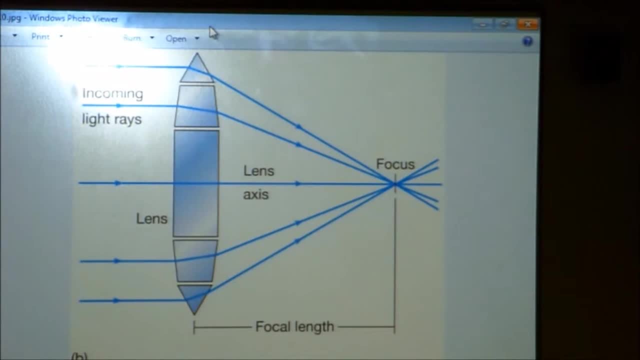 light's seeing it directly. it's going to go straight in and straight out, straight through to the focal point. Down below we have an upside down narrow angle prism and it's going to go straight in and straight out, straight through to the focal point. 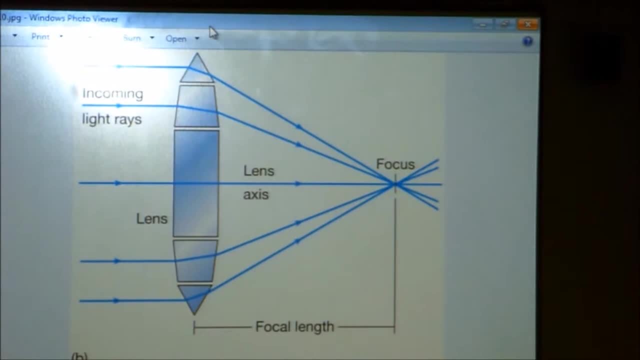 A little bit of deflection in the angle and under that you have an upside down wide angle prism. You get a big angle in the deflection, So all the rays come to the focal point. Now this is really a very cumbersome way of making a lens, getting a whole bunch of 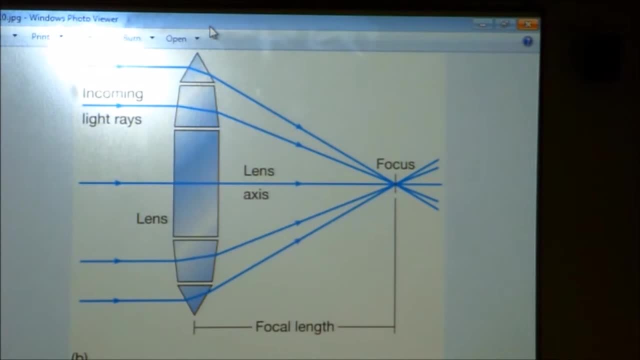 prisms and chopping them up and sticking them together, And it's not very good. Right now. this one's only made of five pieces. Ideally you'd want to do maybe 20, where each one is changing the angle just a little bit, Or maybe a hundred or a thousand, And it becomes. 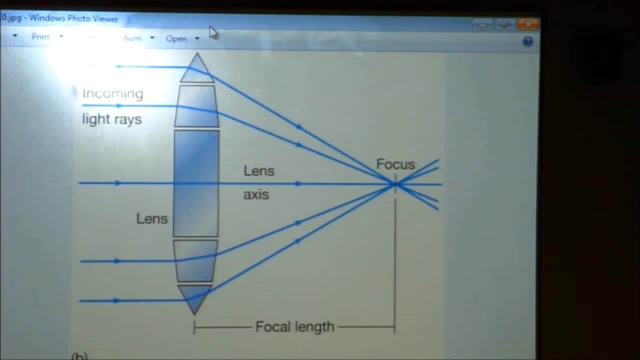 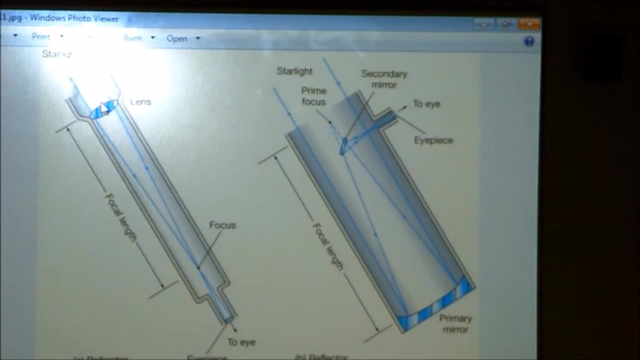 really cumbersome to get all these prisms and chop them up and stick them together. Instead, you can just make a single piece of glass, like you see right here. that is, changing the angle of the surface as you go from the top of the lens to the bottom. So 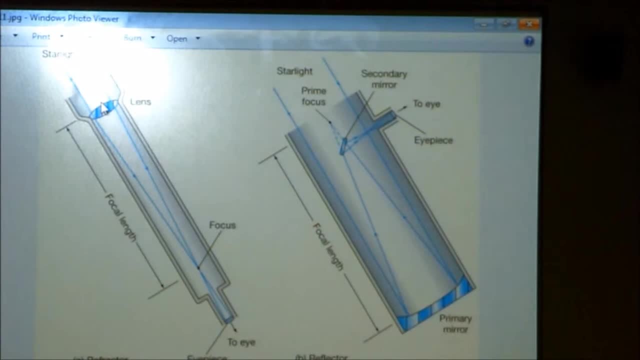 you can make it out of just one piece of glass. You don't have to actually glue a bunch of prisms together. That's just pedagogical to help you understand what's going on. So you all get lenses right, Okay. so here we have our two types of telescopes. We have 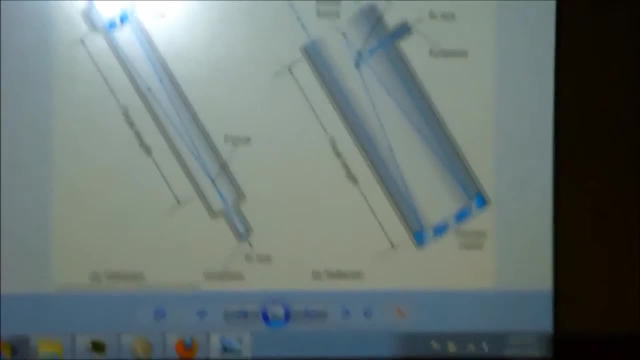 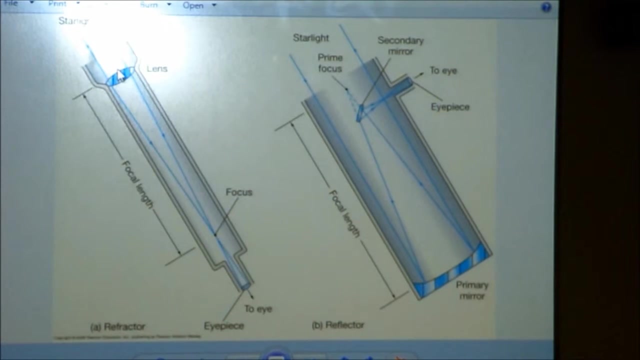 the reflector on the left and it looks like you're at the pirate telescope that you hold up to your eye, And then the reflector on the right. So let's see what's going on here. It's a basic mechanism of two very basic telescopes. We have light coming in starlight. 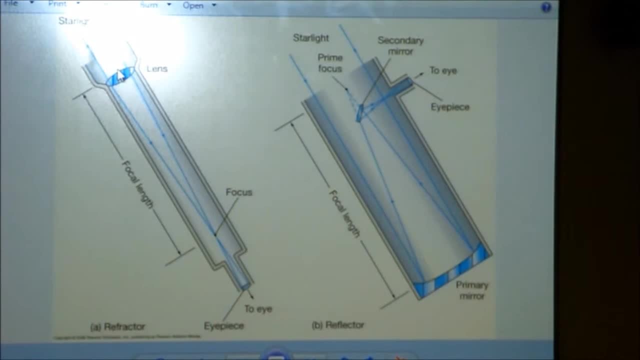 parallel rays, because the object is so far away- enters the lens and it's focused down to the focal point, which is marked right there Here. And in this case the focal point is in the tube. And you might think, boy, that's strange. Isn't that where I'd want? 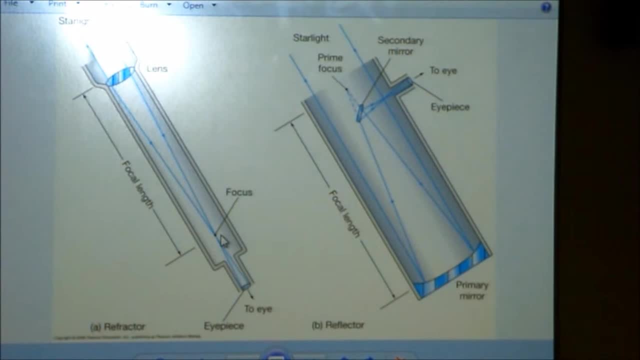 to stick my eye. That's the focal point. Right there is where the image forms. But instead of sticking your eye there, it lets it continue, go out of focus. hit another lens, the eyepiece, just a little lens, which will then make the rays parallel again. 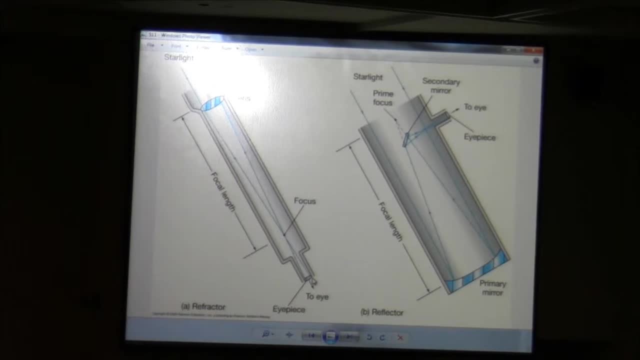 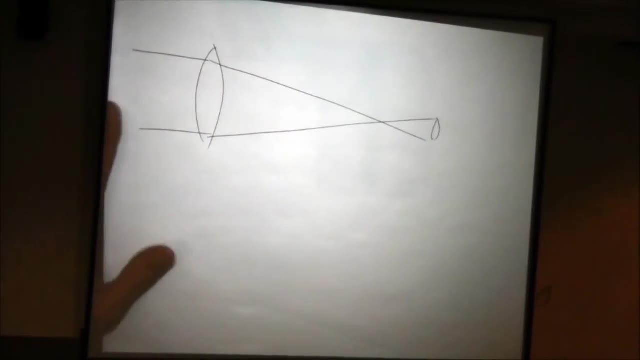 Maybe I'll draw it myself. So you've got the big lens on the end of the tube and then the rays come in. they go past the focal point then through a little lens, usually about the size of the human eye, and it comes out parallel. And this is the only place in what 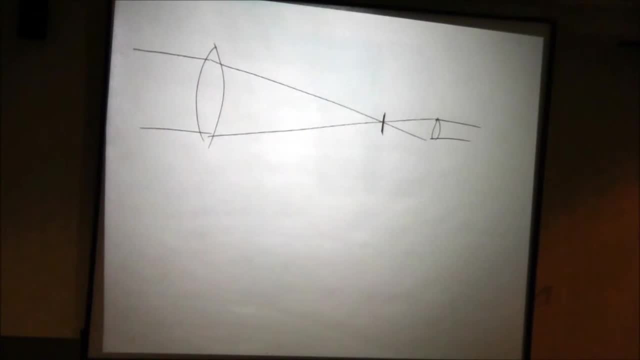 you see here anyway where it's in focus. So why would we do that? Why would we want the rays to come out parallel and not at a focal plane? Any idea. It has to go through the lens of your eye. This is not the full telescope. If you're using your eye now, if 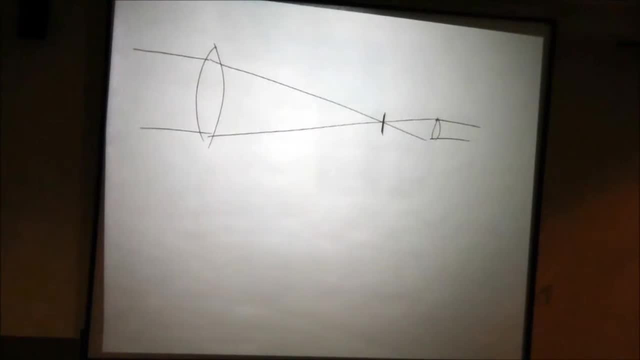 you're using a digital camera, you're going to be able to see what's going on in your eye. But if you're using a digital camera, you would not do this. You'd stick the digital camera right here. You'd saw off the end of the telescope. you'd stick your digital camera. 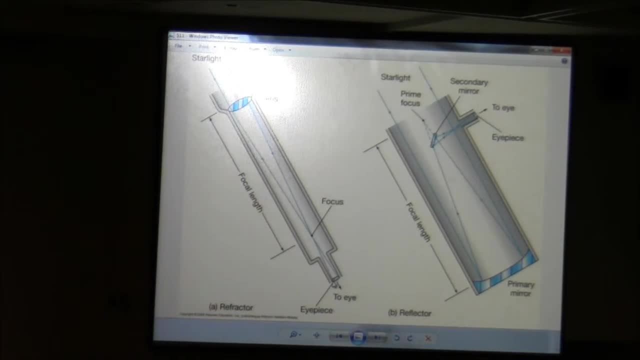 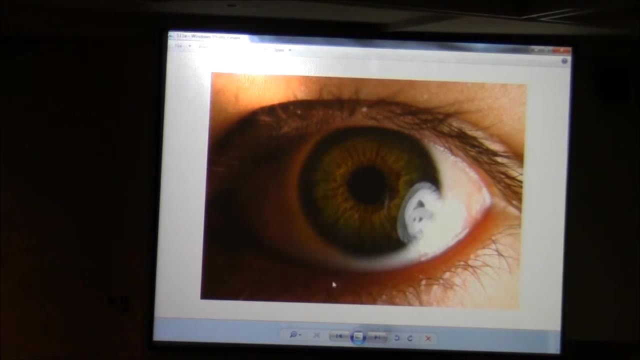 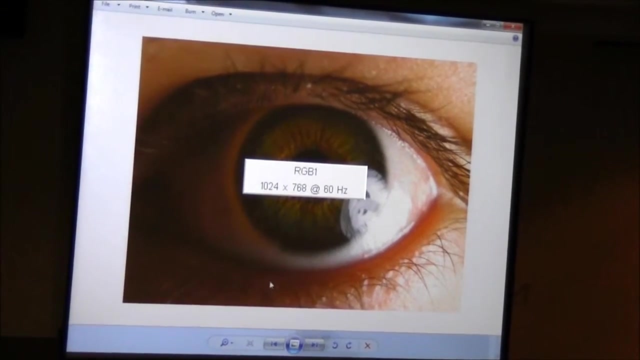 right here, But if you're going to hold it up to your eye like a pirate telescope, then your eye is alsoit's a little freaky actually. Oh, I gotta try this. I've never done this before. Let's see here. Is that like extra freaky, Both of them looking at you, Yeah. 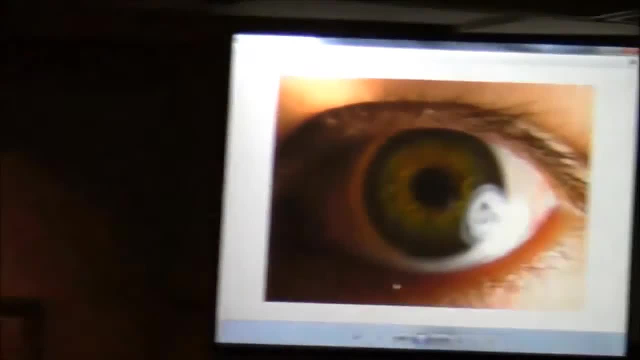 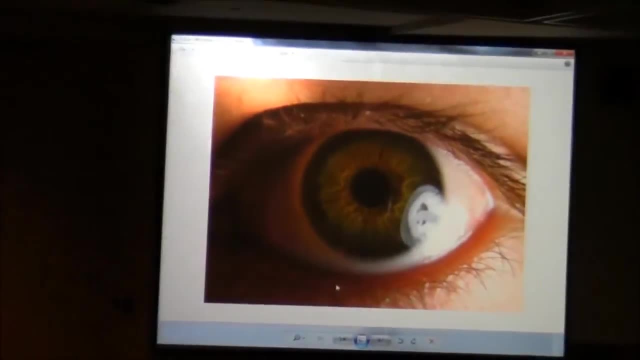 that's cool. Okay, Back to the dot cam. So the eye is a telescope And it is a pretty cool telescope. It's a biological telescope And so the light is going in just in that central part And you can change how much light goes in or how much light is blocked, depending upon what 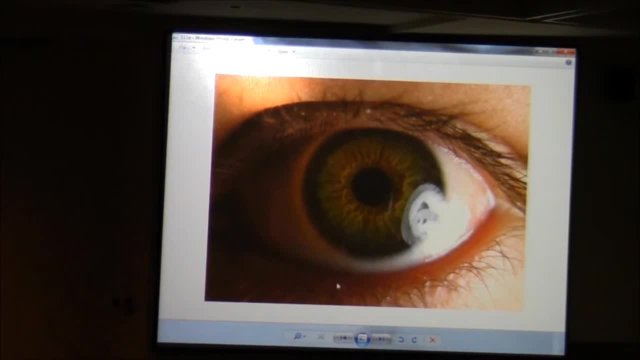 you're looking at. If you're looking at something bright, the eye restricts, only a little bit of light goes in. Or if you're in faint conditions, it opens up, your pupil dilates and a lot of light goes in. So it has that kind of self-control on it, because your detector can only take. 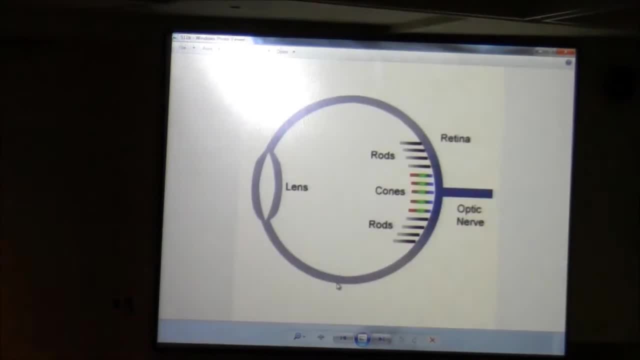 a particular light range, and so it helps out that way. And here's the image from before. Before we talked about the cones and rods of the eye, but the entry point there is a lens. It's a biological lens. It's refracting the light. So if you look at something far 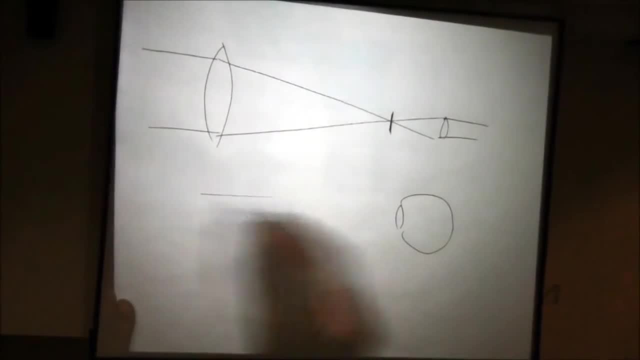 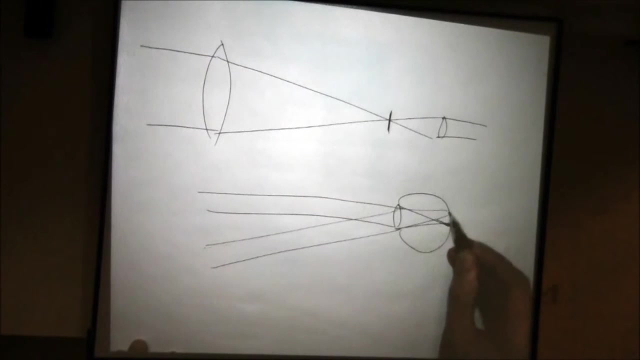 away. the idea is they're coming and the focal point is on the back. Not here, but on the back is where you have your cones and your rods. Something's coming from down below. it will image higher up in the back of your eye, So you have this kind of curved focal. 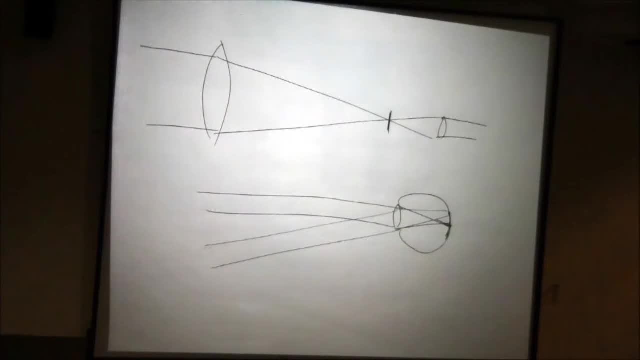 plane in the back of your eye. In fact, in dark conditions, when you're using your rods, your peripheral vision's better for that reason, because on the main axis you don't have rods, you have cones. So in dark conditions, whatever's right in front of you, it's actually harder. 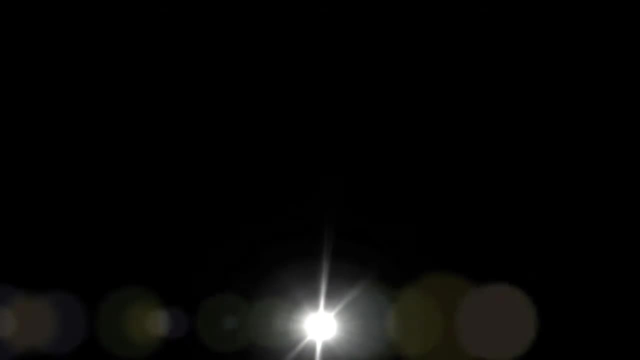 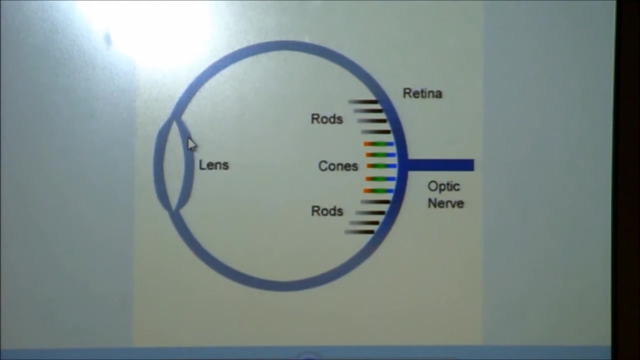 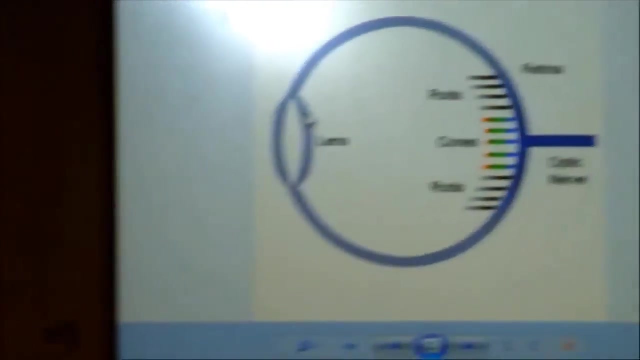 to see than stuff off on the side. It's kind of a nifty telescope because it's a telescope that can change its focus pretty easily, And most of the telescopes astronomers make, they're designed to be focused on something really really far away. If you try to look at something nearby, you'll be out of focus. 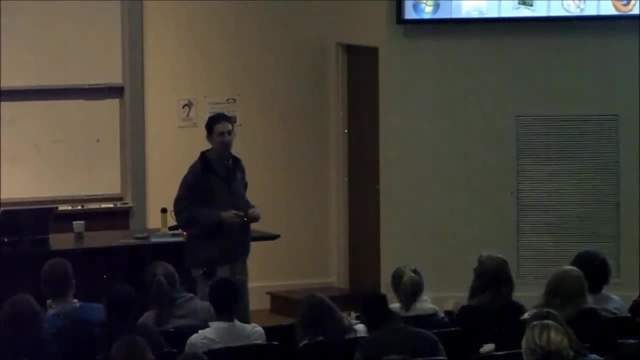 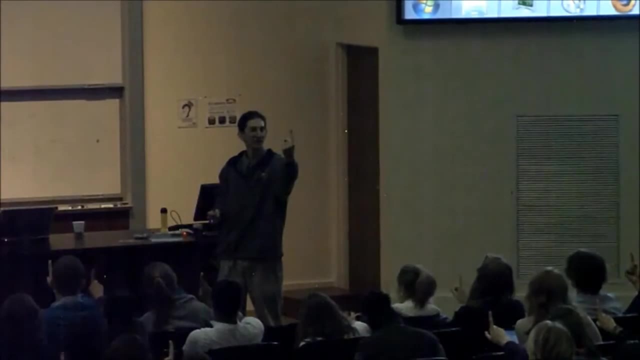 But the human eye is adaptable. There are muscles that attach to the lens and can bend the lens. I can go ahead and do the thing with the finger again. Take the finger really far from your head and focus on it, So you're no longer focused on the wall but you're focusing on the wall with your finger. Move that finger closer and closer. You can focus at a whole bunch of different distances until there's a point that it hurts. That's the limit. It's the strength of the muscles attached to your lens, trying to warp it, bend it to. 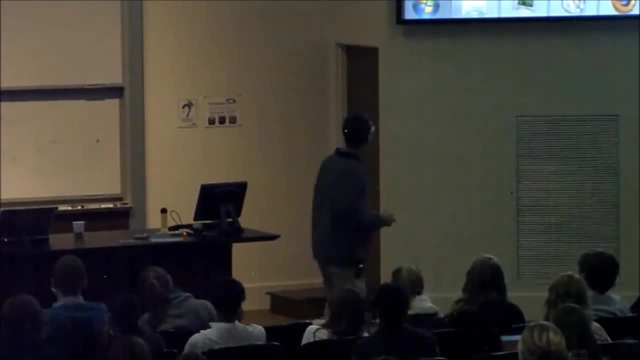 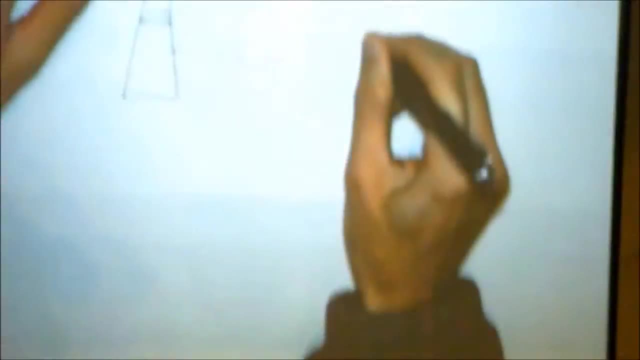 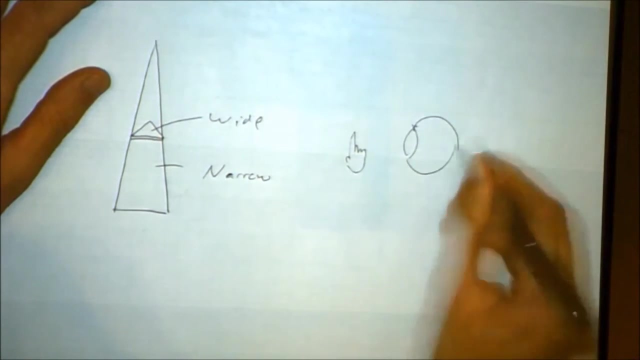 change the focusing properties. So it's a telescope that can focus nearby. Here's your finger- Yeah, that's the right finger if you want to make sure. And here's the eye And the light that's coming from your finger. it's actually bouncing off your finger, Your. 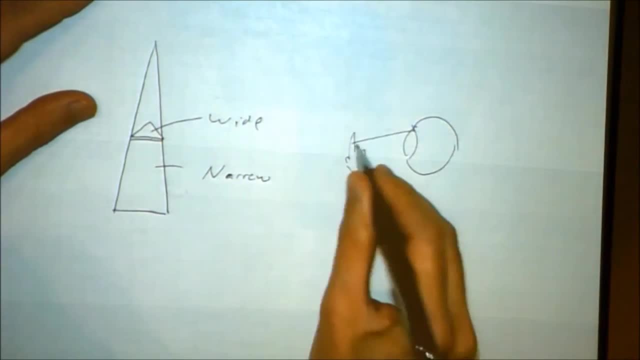 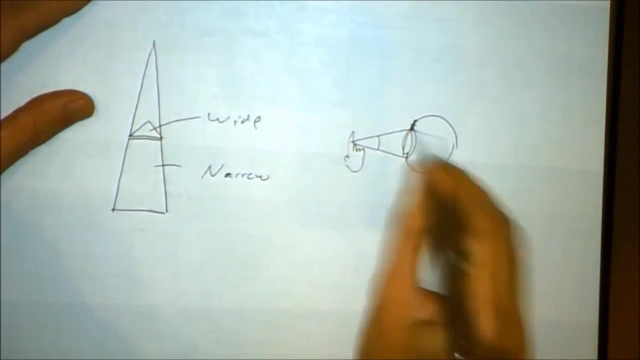 finger's not emitting light, It's not coming in in parallel rates. There's an angle there, But the muscles can stretch and pull the lens tighter such that it still will focus here. Where astronomical telescopes? they're designed only for things far away- The human eye also. 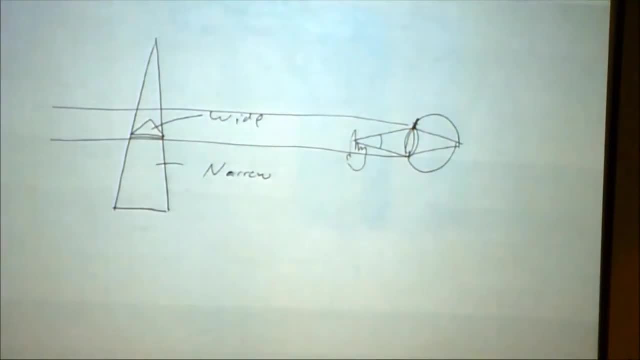 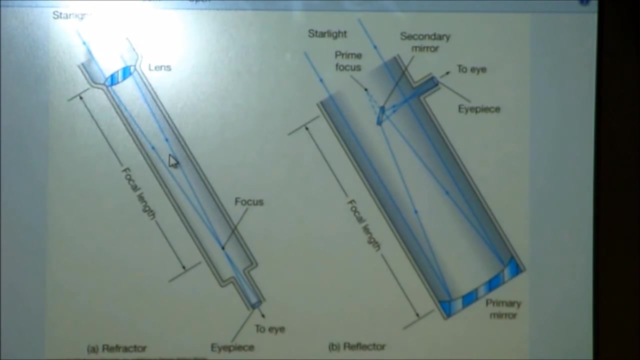 works for things far away too. That's kind of the natural relaxed position: seeing things far away. Okay, back to this image. On the right we have the reflecting telescope. This is just one of many possible different configurations. Light comes down, bounces off the primary, It would. 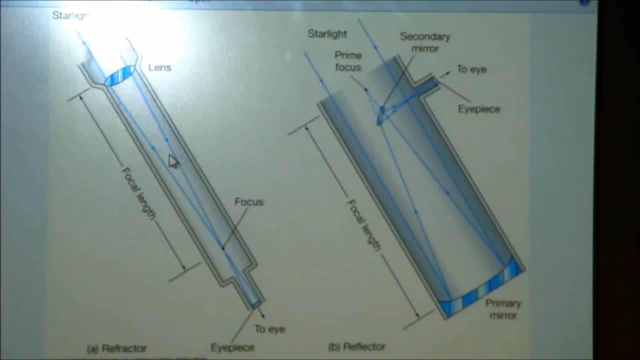 go to a point called prime focus. Again, there's no point in sticking your eye there, because the eye wants the light to be coming in at least roughly parallel. So it doesn't have to be perfectly parallel. The human eye has that flexibility, But the closer we make it parallel, 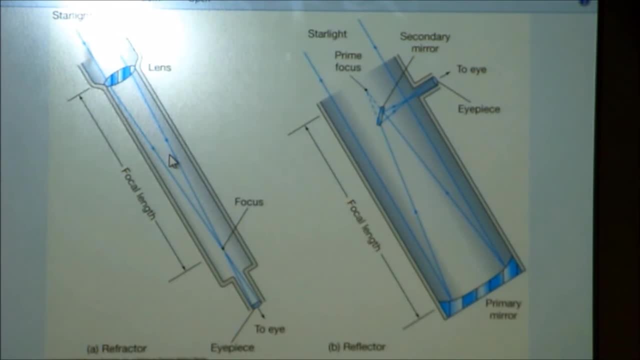 the better. So one way to do this would be to let the light go through prime focus and then stick a lens there, and then stick your eye on the lens, but your head's then blocking the telescope. That's a problem. So here's one possible configuration. You have a little. 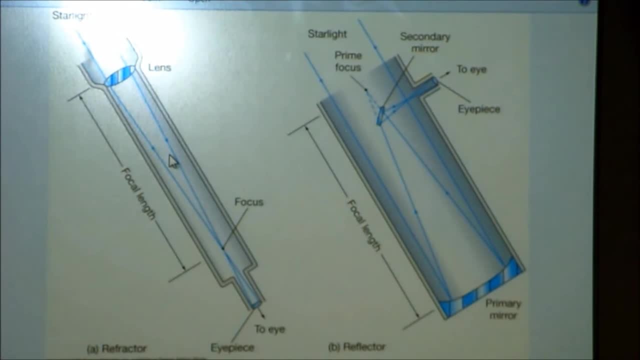 mirror there. Before it hits the focal point, it takes the rays and bounces them off to the side. This is called a secondary mirror. In this case it's a flat mirror. Bounces off to the side. The focal point would be here. You go past focus into an eyepiece.